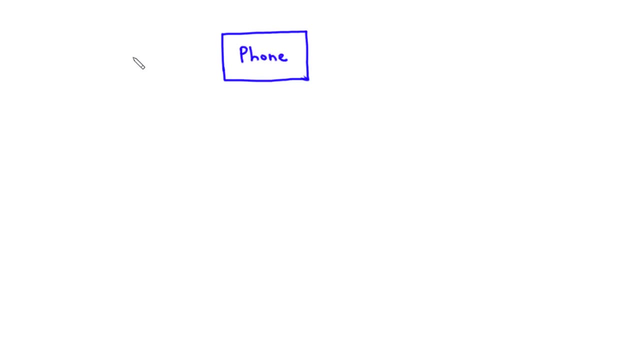 a third party at 500 Ghana cedis And then later you sold the phone at 550 Ghana cedis to a friend. Now the amount that you used in buying the phone is called the cost price and the amount that you sold the phone is called the selling price. 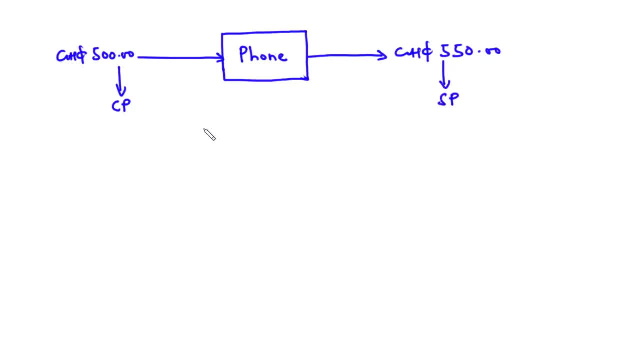 So let's assume you bought a phone from a wholesaler, a manufacturer or, better still, a third party at 500 Ghana cedis to a friend. So what do you think? Did you make a profit or a loss Since the amount you sold the phone? 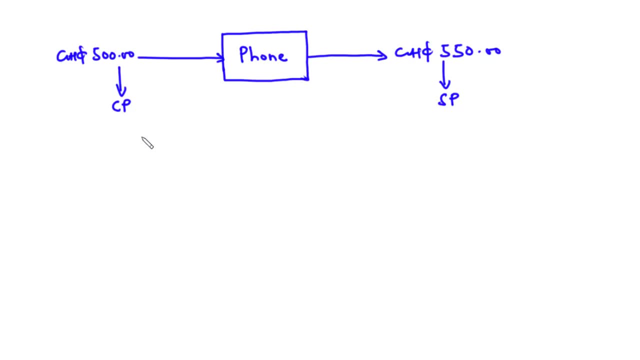 is higher than the amount in which you used in buying the phone, we say that you made a profit. Ok, so how do we find the profit? The profit is basically the selling price minus the cost price. So in this case we have the selling price to be 550 Ghana cedis. 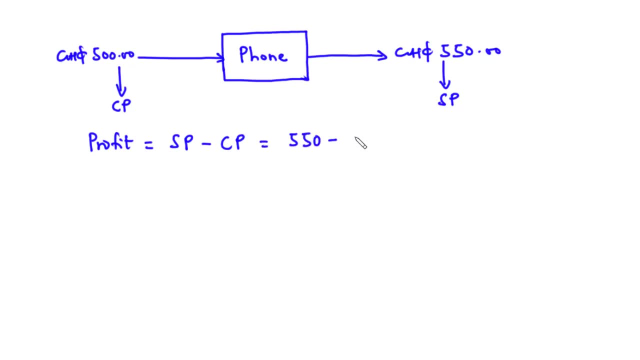 50 Ghana cds and the cost price to be 500 Ghana cds. so the profit is basically 50 Ghana cds. so this is the profit that you made. now let's consider this to be our first case now, assuming that after buying the phone for 500 Ghana cds, you sold it at 400 Ghana cds. 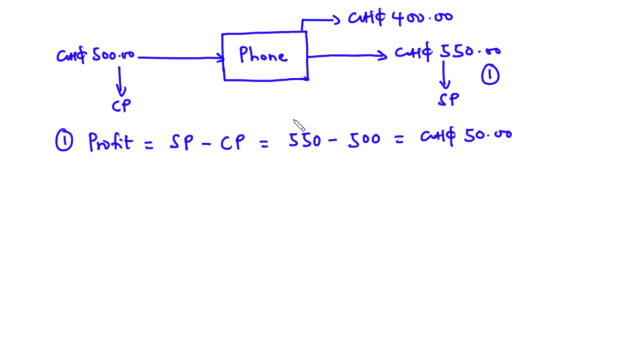 this time because the selling price is less than the cost price, we say that you made a loss. so for the second case we are going to look for the loss which is equal to the cost price minus the selling price. we have the cost price to be 500 Ghana cds and the selling price 400 Ghana. 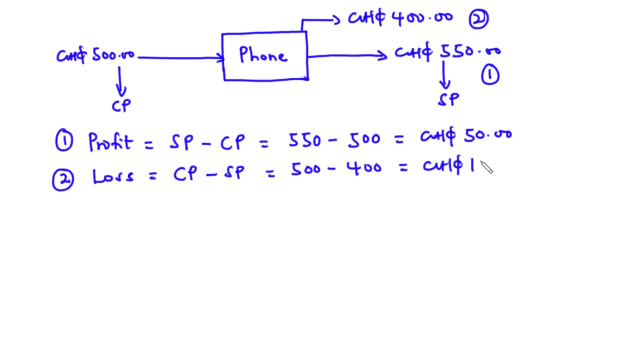 cds. the difference is 100 Ghana cds, So this is the loss you made. So in the first case you had a profit, which is 50 ganassidis, And in the second case you had a loss of 100 ganassidis. 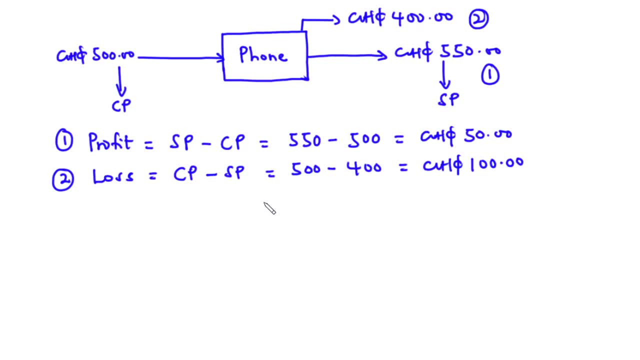 Now some questions require that you calculate or find the profit percent or the loss percent. The profit percent is giving us the profit over the cost price times 100%. So for the first case we have the profit to be 50 ganassidis. 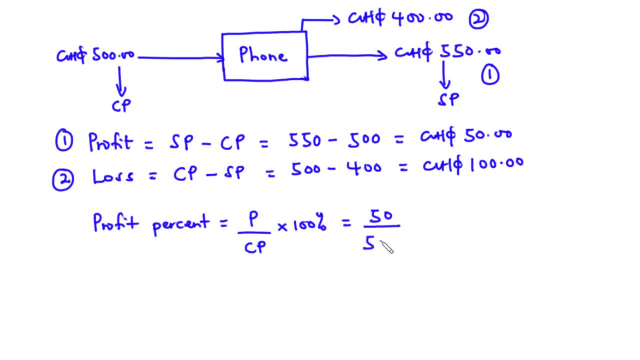 So 50 divided by the cost price, 500, times 100%, 50 goes here once into 50. So 500, 10 times 100 divided by 10 gives 10.. So we have the profit percent to be 10.. 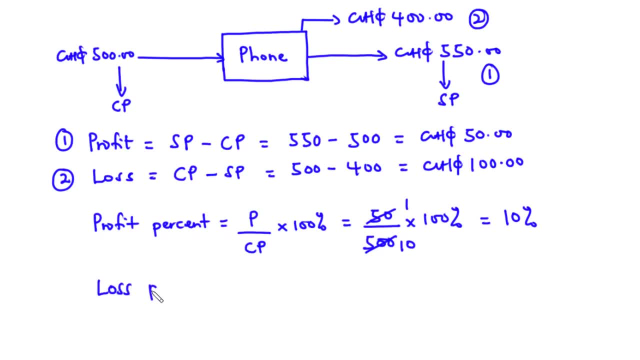 Now to the loss percent. The loss percent is also given by the loss over the cost price times 100%. So we had the loss to be 100 divided by 500 times 100.. 100 goes here once into 500, 5 times. 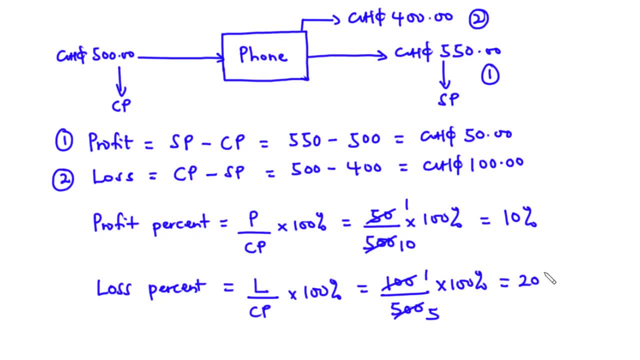 100 divided by 5 gives 20.. So we have 20%. So basically, profit and loss are often given as percentages of the cost price. So always the cost price is fixed and remains at the denominator. Now let's take a look at some other equations. 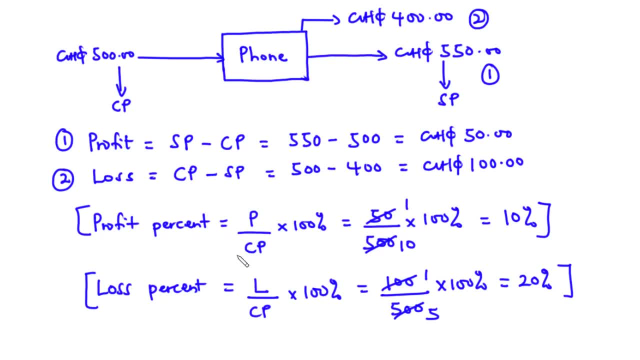 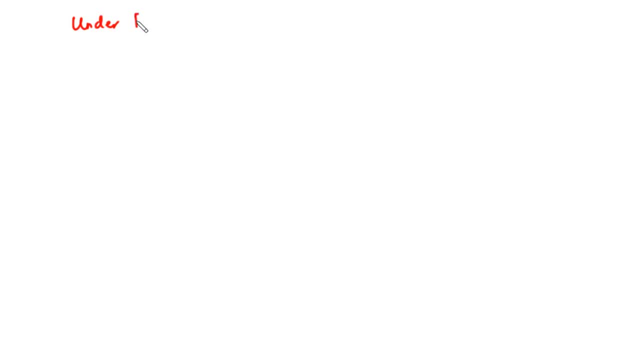 Involving profit, loss, profit percent and then loss percent. So under profit, Under profit. First of all, the profit is equal to the selling price minus the cost price. The profit percent is equal to the profit over the cost price times 100%. 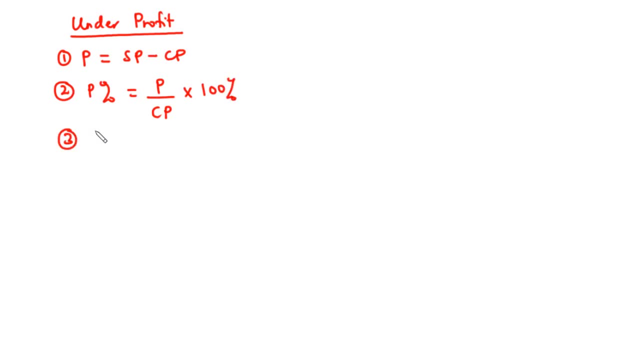 3, We have the cost price equals 100 over 100 plus the profit percent times the selling price. And then for the last one, we have the selling price equals 100 plus the profit percent over 100 times the cost price Involving profit loss, profit sales. 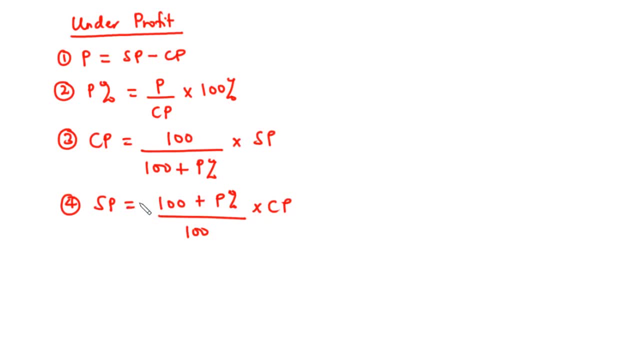 100 divided by cash, Mmm. Now you don't need to keep all these formulas in mind, especially that of the cost price and the selling price. Now all you need to know is that, under profit, the cost price is equivalent to 100 and the selling price is equivalent to 100 plus the profit percent. 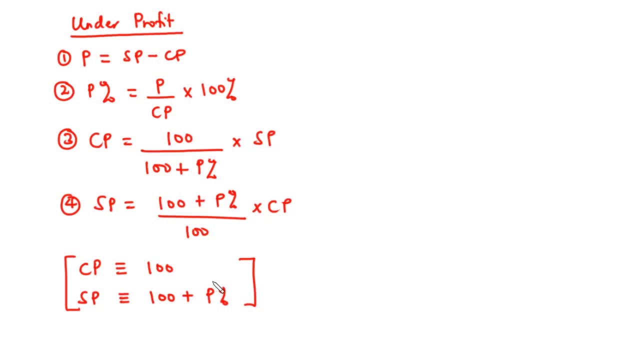 So, knowing this offhand, you can use simple ratio and proportion to determine the cost price and the selling price. Now let's consider under loss. So under loss, we have loss to be equal to the cost price minus the selling price. 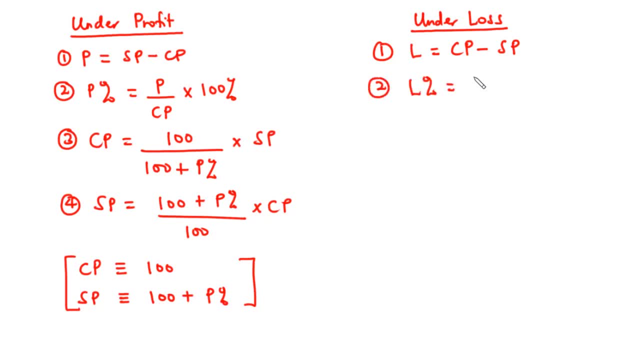 We have the loss percentage to be equal to the loss over the cost price times 100%. Three, we have the cost price to be equal. So, under loss, we have the cost price to be equal to 100 divided by 100 minus. this time the loss percent times the selling price. 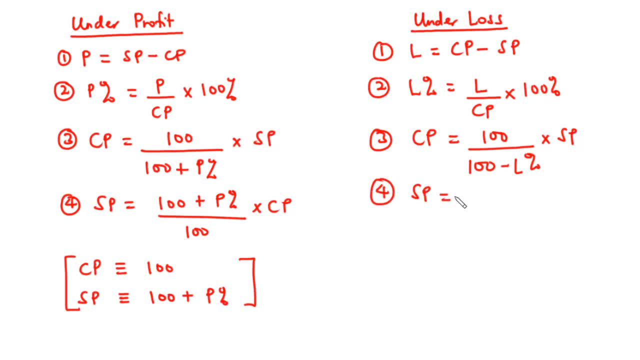 And also for the last one we have, the selling price equals 100 minus the loss percent, over 100 times the cost price. So also under loss the cost price is equivalent to 100.. And the selling price is equivalent to 100 minus the loss percent. 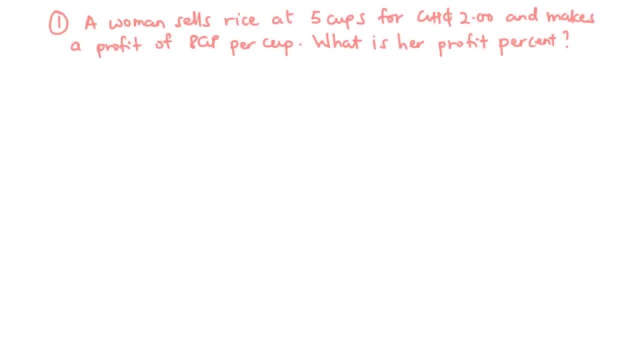 So let's move ahead and try some examples. So let's take our very first question. A woman sells rice at five caps for two Ghana cedis and makes a profit of eight Ghana pesos per cap. What is her profit percent? A woman sells rice at five caps for two Ghana cedis and makes a profit of eight Ghana pesos per cap. 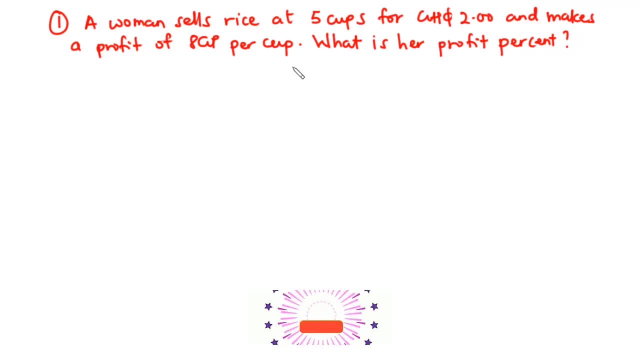 What is her profit percent? So now let's solve this question together. So from the question we are told that the woman sells rice at five caps for two Ghana cedis. So the selling price of the five caps is two Ghana cedis. 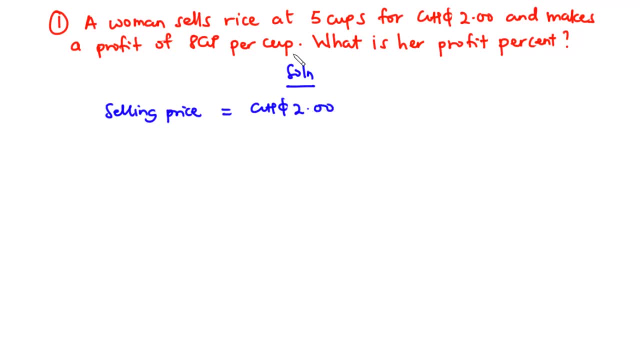 And then she makes a profit of eight Ghana pesos per cap. so profit per cap is 8 Ghana pesos, which is equal to. you want to divide 8 by 100, so that is 0.08. okay, so you have 0.08 Ghana cds. so this is the profit per cap. now she sold five caps, so we are. 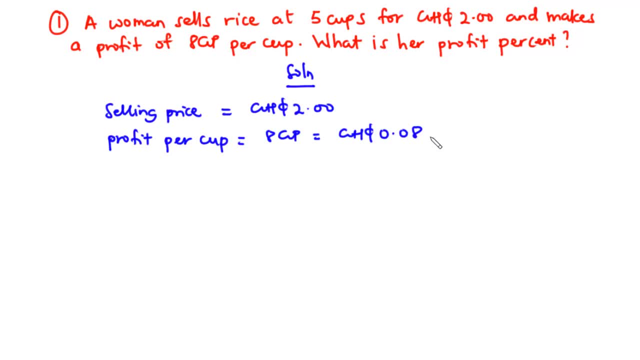 going to multiply five by 0.08 to obtain the profit she made after selling the five cups. so profit for five cups is equal to 0.08 times 5, which gives us 0.40 Ghana cds. now we are asked to find her profit percent. 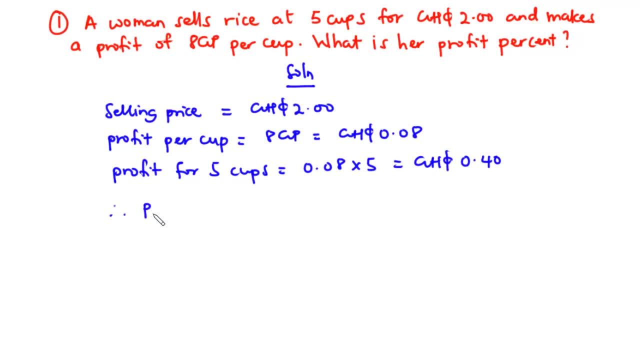 so profit percent. profit percent is given by the profit over the cost price times 100 percent. now we know your profit but we don't know the cost price. so to find the cost price, cost price is given by the selling price minus the profit. so we have the selling price to be. 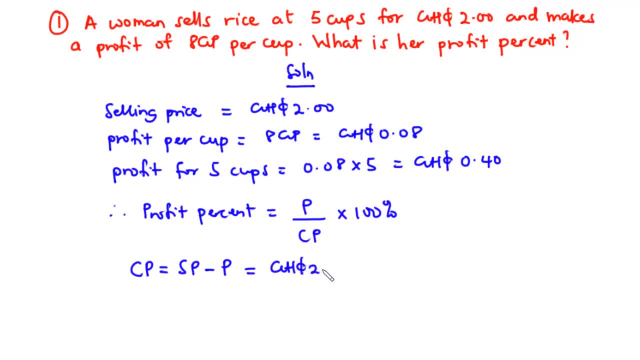 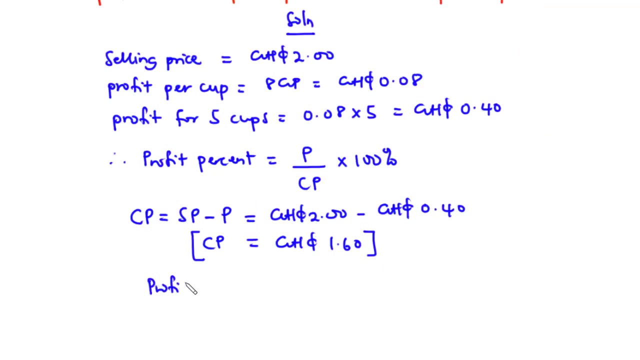 two Ghana cds minus the profit, which is zero point four Ghana cds. so we have the cost price to be one point six, zero Ghana cds. so this is the cost price. now using this value we can find the profit percentage or the profit percent. so the profit becomes profit is 0.40 divided by a cost price 1.60 times 100 percent. 0.40 times 100 gives 40. 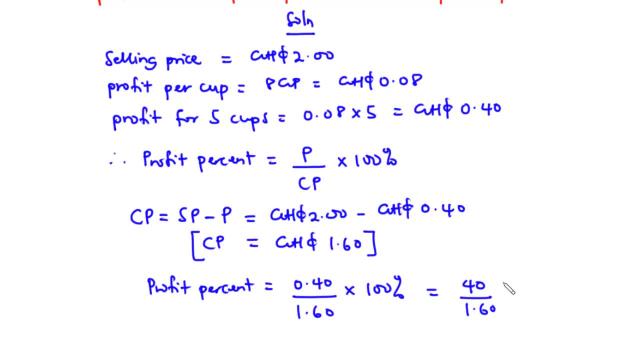 and then divided by 1.60, which is equal to 25 percent. so it means that the profit percent is equal to 25 percent. so this is the profit percent that she made. now let's move on to the next question. so question two: a woman sold an article for four ghana cities. 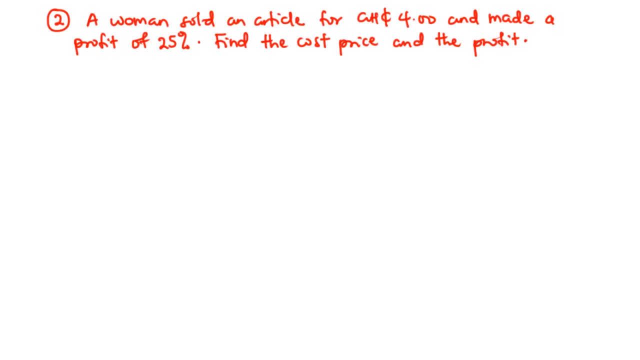 and made a profit of 25 percent. find the cost, price and the profit. a woman sold an article for four ghana cities and made a profit of 25 percent. find the cost, price and the profit. so for this question we are told that the woman sold an article for four ghana cities. 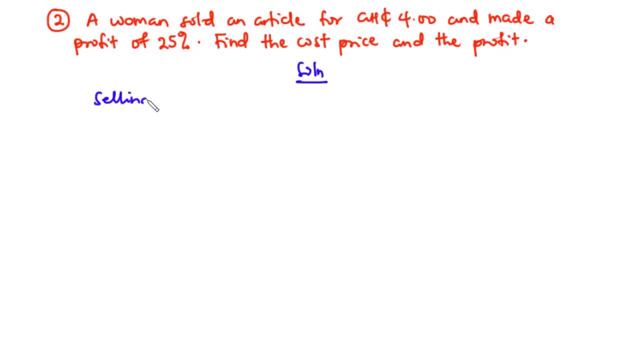 so we have the selling price to be four ghana cities and then she made a profit of 25 %. so that is the profit percent is 25. so you are going to find a cost price and the profits. so first of all let's find the cost price. so under profit, we said that a 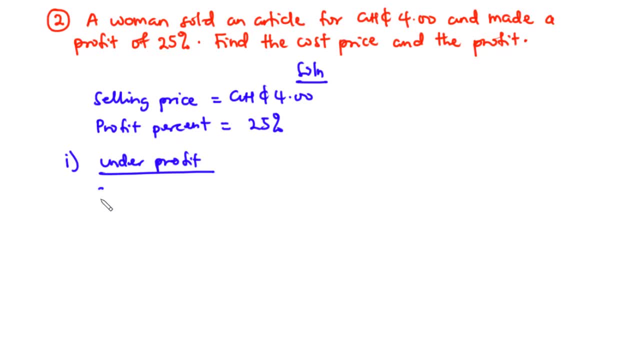 The cost price is equivalent to 100 and the selling price is equivalent to 100 plus the profit percent. Now here we have the selling price and the profit percent, So we can use simple ratio and proportion to determine the cost price. Now we have the selling price to be 4 Ghana CDs. 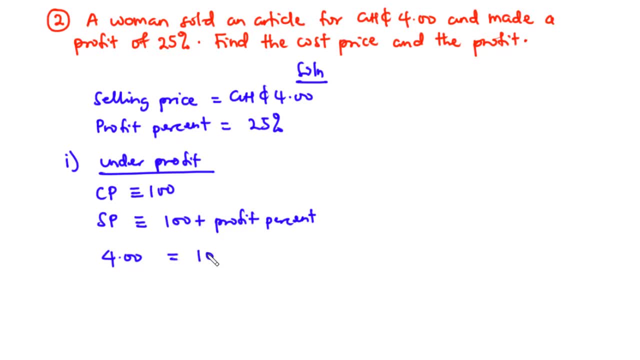 So 4 CDs equals 100, plus the profit percent is 25.. So plus 25. Now we have the cost price to be equal to 100.. Now if less, more divide, So to find the cost price, the cost price is basically going to be: 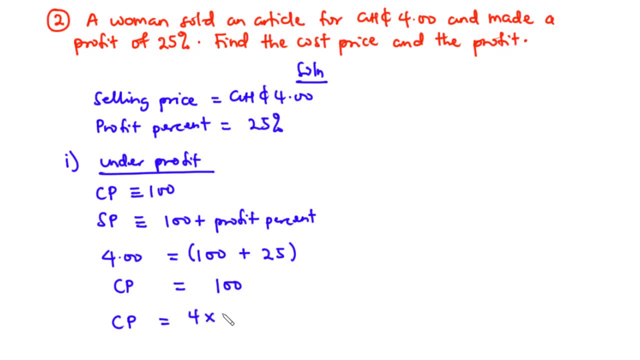 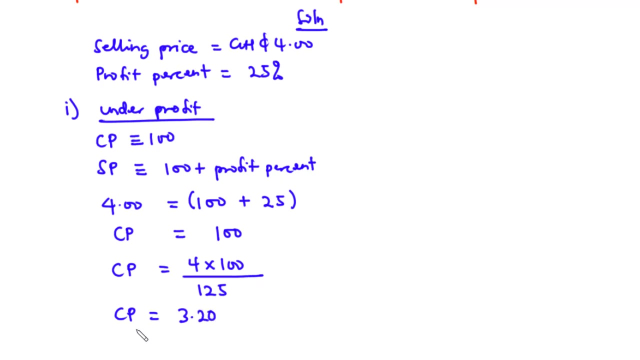 4 times 100 divided by 125.. So the cost price is equal to 3.2, 3.20, which is equal to 3 CDs, 20 Ghana Pesos. So this is the cost price. Now let's find the profit. 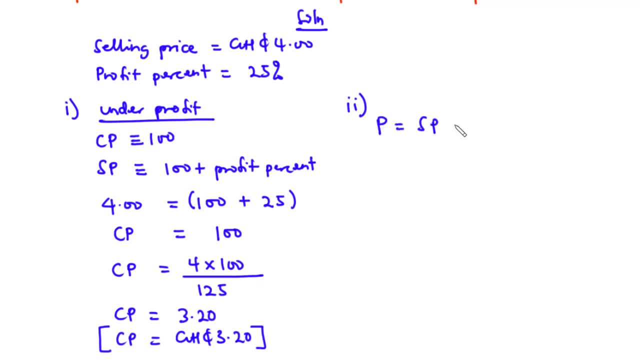 So the profit is given by the selling price minus the cost price. We have the selling price to be 4 Ghana CDs and the cost price to be 3.2 Ghana CDs. So when you subtract this from that you have 0.80, which is 0.80 Ghana CDs or, better still, 80 Ghana Pesos. 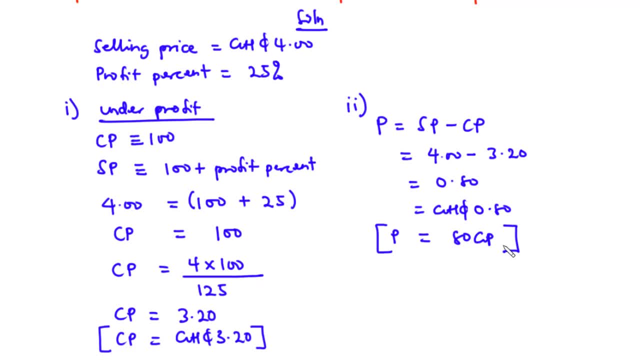 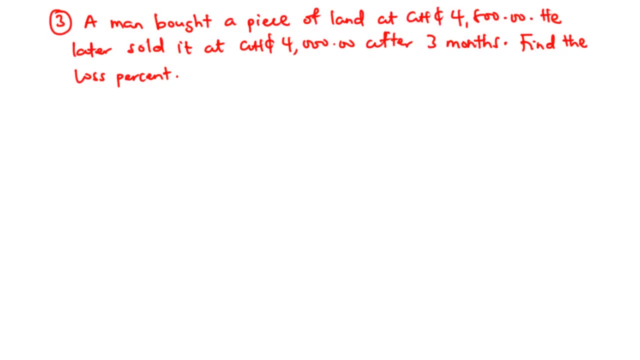 So this is the profit. A man bought a piece of land at 4,800 Ghana CDs. He later sold it at 4,000 Ghana CDs after 3 months. Find the loss percent. Find the loss percent. So the man bought a piece of land at 4,800 Ghana CDs. 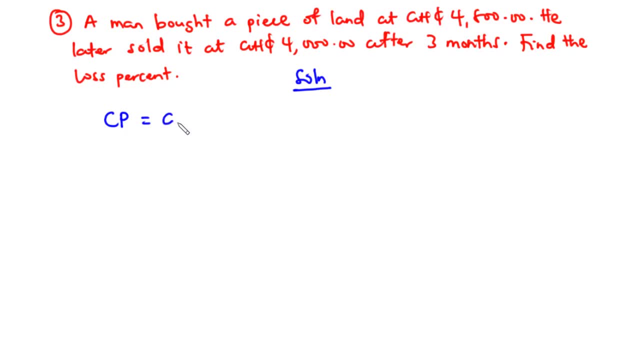 So the cost price is 4,800 Ghana CDs. So the cost price is 4,800 Ghana CDs. So the cost price is 4,800 Ghana CDs. So the cost is 4,800 Ghana CDs. So the cost price is 4,800 Ghana CDs. 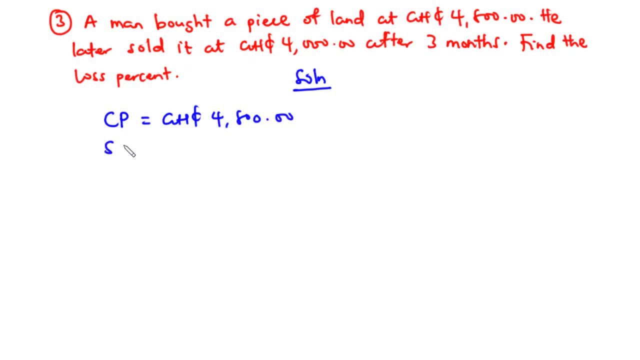 And then he sold it at 4,000 Ghana CDs. And then he sold it at 4,000 Ghana CDs. So that is the selling price: 4,000 Ghana CDs After 3 months. Now we are going to find the loss percent. 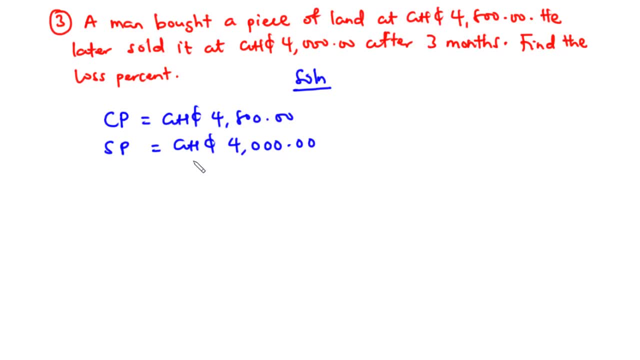 Now the loss percent is given by the loss over the cost price times 100%. So we need to find the loss, The loss. the loss is given by the cost price minus the selling price. we have the cost price to be four thousand eight hundred Ghana cities and then the selling price. 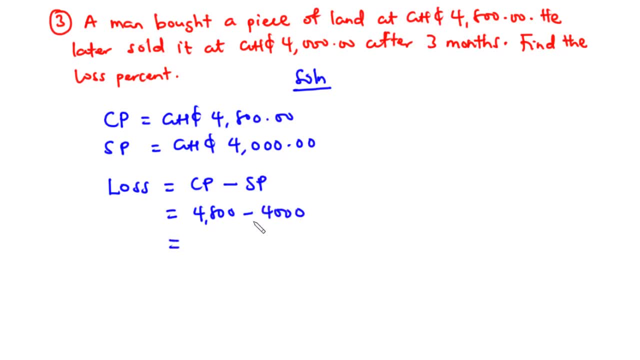 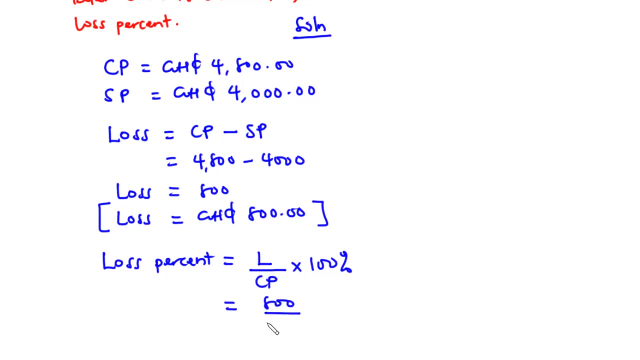 to be four thousand Ghana cities. so four thousand. eight hundred minus four thousand gives eight hundred. so this is the loss. the loss is eight hundred Ghana cities. now let's find a loss percent. so the loss percent is given by the loss over the cost price times 100%. so we have lost to be 800 divided by four.